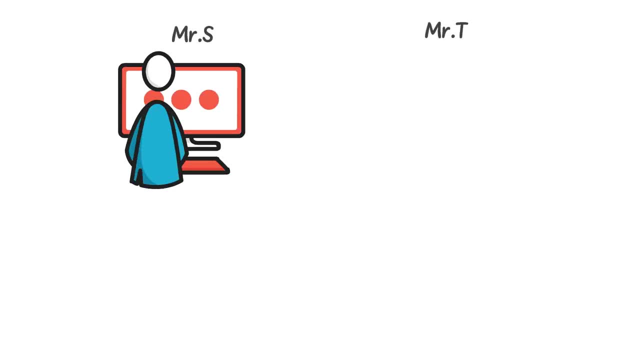 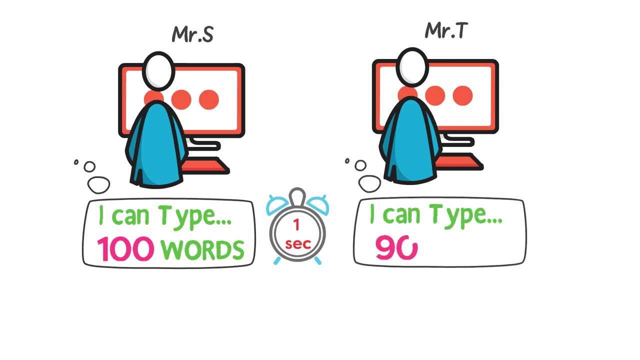 in 1 second. Thirdly, consider Mr S and Mr T. Let Mr S can type 100 words in 1 second And Mr T can type 90 words in 1 second. Can you guess the typing frequency of Mr S and? 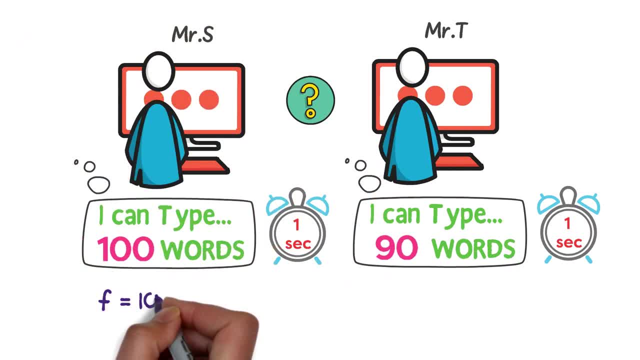 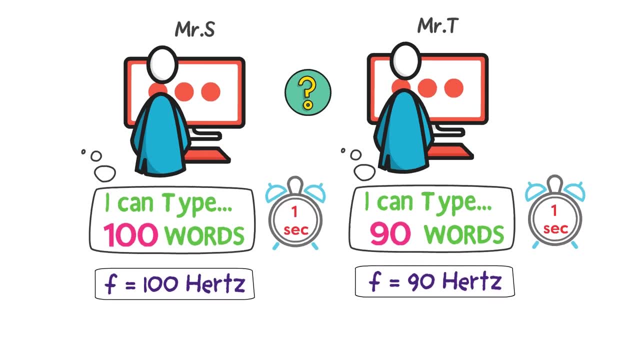 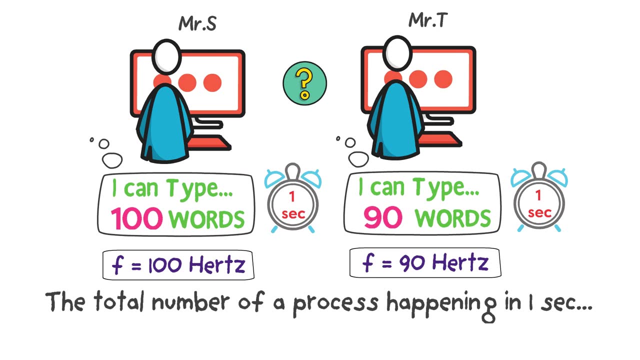 Mr T. Well, the typing frequency of Mr S is 100 hertz and the typing frequency of Mr T is 90 hertz. Thus we define frequency as the total number of a process happening in 1 second is called frequency. Usually, frequency describes the total number of a process that 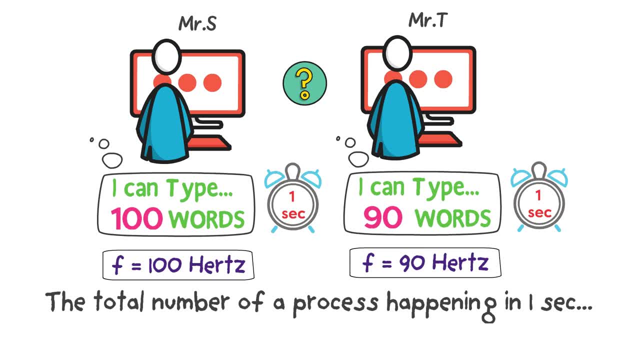 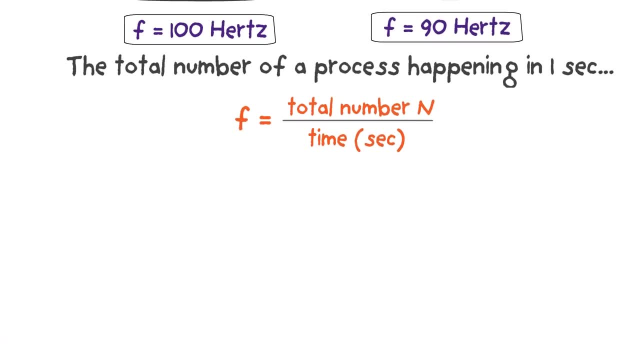 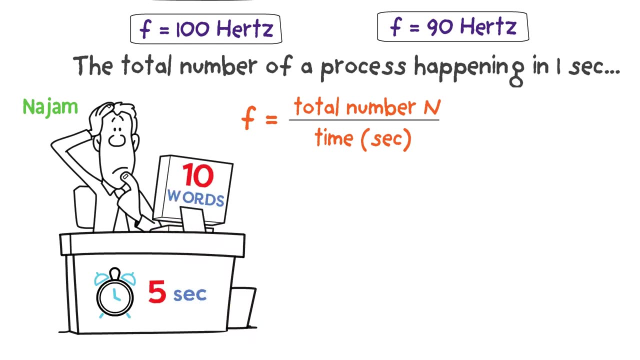 is repeating itself over the time. The formula of frequency is: f is equal to total number, n upon time, n second. For example, consider Mr Najm. He can type 10 words in 5 seconds. What is the typing frequency of Mr Najm? Well, we know that f is equal to 10 words. 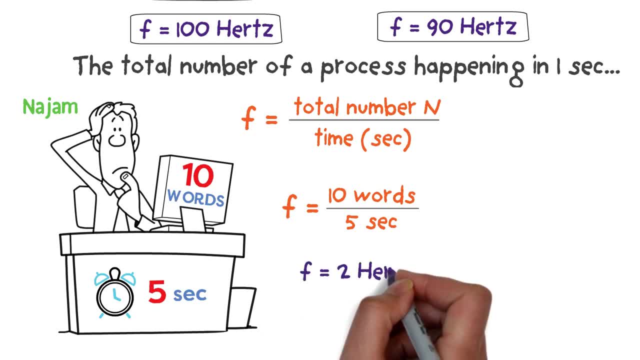 upon 5 seconds. So the typing frequency of Mr Najm is 2 hertz And he is 90 hertz. So the typing frequency of Mr Najm is 2 hertz And he is 90 hertz. 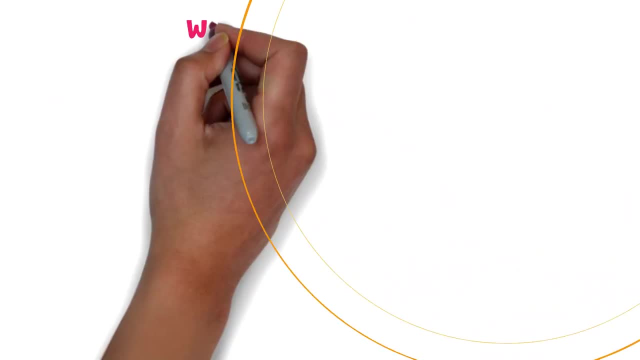 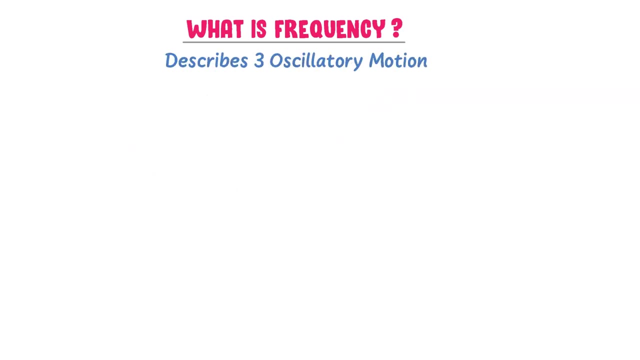 He is not a suitable person for typing job. Now, what is frequency and physics? Usually, frequency describes three oscillatory motion and physics. For example, consider light wave, circular motion or SHM and sound wave To understand the concept of frequency and physics. 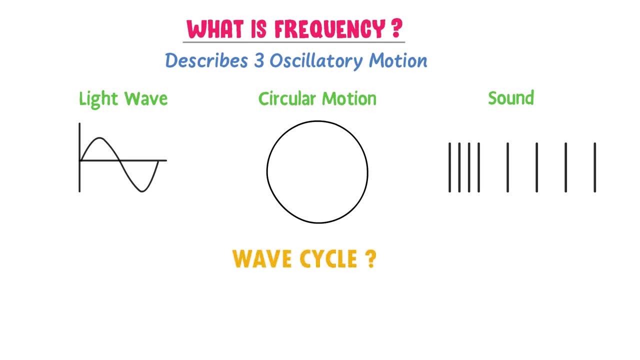 you must understand the concept of wave cycle. For instance, in transverse wave or light wave, one crust and one trough make up the wave cycle. For instance, in transverse wave or light wave, one trough makes one cycle And circular motion. consider a point A. If 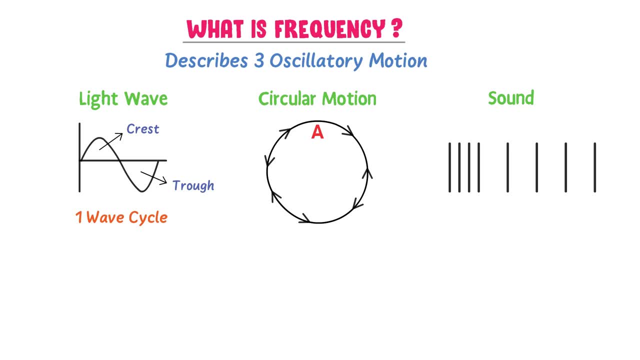 a body moves from point A and come back to point A, we say that one cycle is completed And longitudinal wave or sound wave, one compression and one rarefaction forms one cycle. Thus, in physics we define frequency as the total number of cycles n completed in one second.